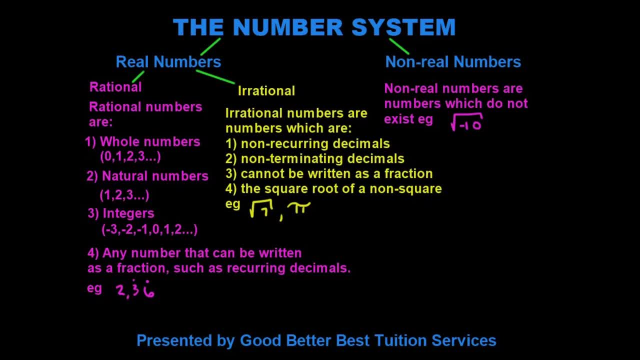 The number system is broken up into real numbers and non-real numbers. So non-real numbers are numbers which do not exist. So that would be, for example, the square root of a negative number. Those numbers are not real or they are imaginary. Then we have real numbers Now. real numbers are: 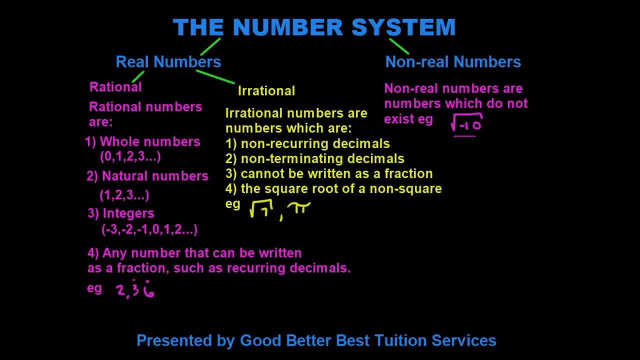 broken up into two sections. They are rational numbers and they are irrational numbers. Rational numbers are numbers which are whole numbers, For example zero, one, two, three Natural numbers. they are your counting numbers. When you start counting, you start counting at one, You don't start counting at zero. So natural numbers are one- two. 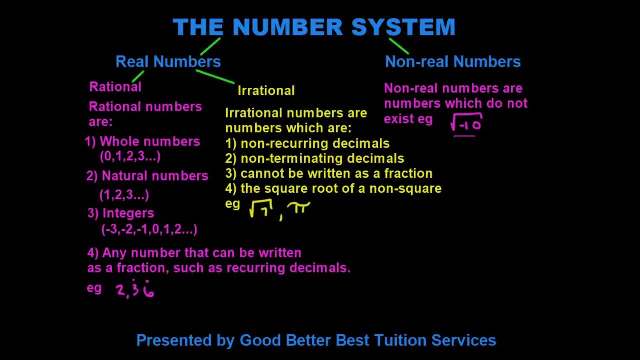 three and so on. Integers: they are your negative and positive whole numbers. Okay, there have to be whole numbers. And then any number that can be written as a fraction is also regarded as a rational number, such as recurring decimals. For example, two comma three, six recurring Those. 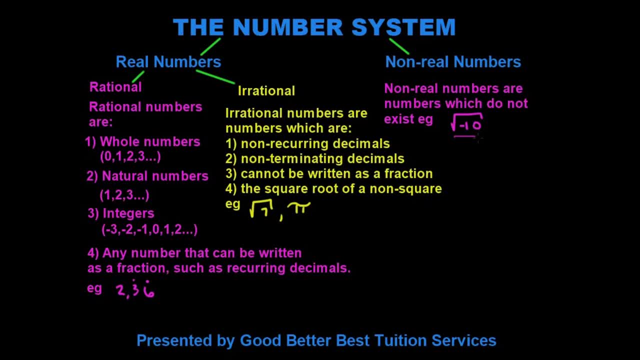 two little dots on top. they mean that that number is recurring. For example, a third is also a recurring number, because if you type it into your calculator, what do you get? You get naught comma three, three, three, three, three. It's a recurring decimal, Okay. but even a number such as a half, 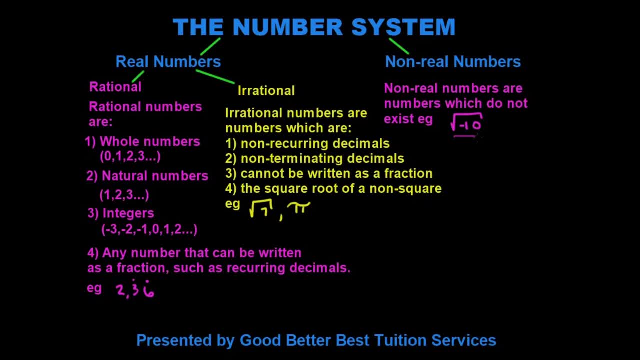 or three quarters. They are fractions, So they are also regarded as rational numbers. Irrational numbers are numbers which are non recurring decimals. In other words, there's no repetition in those decimals. The numbers do not repeat Non-terminating decimals. Those are the numbers which. these are the numbers that do. 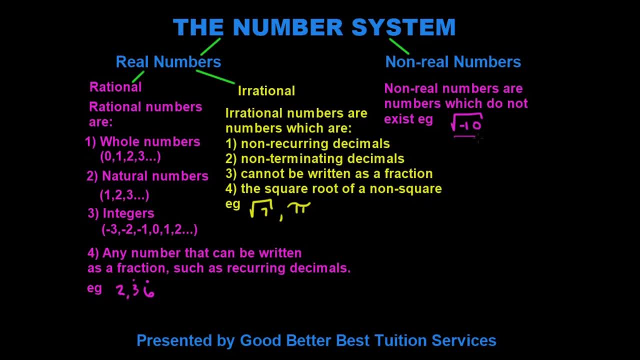 not end. They fill up your entire calculator screen and they cannot be written as a fraction. And then the square root of a non-recurring decimal. So the square root of a non-recurring decimal is one square, For example the square root of seven. That's an example of an irrational 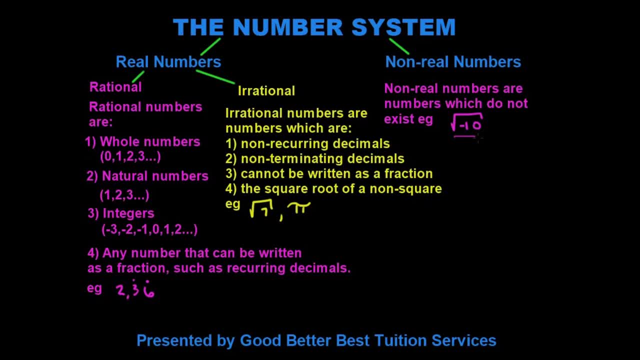 number Pi is also the an example of an irrational number. Okay, you've used pi in when you did area and perimeter, So you should be familiar with it. What I'd like to do now is go through an exercise which I've done with my own learners, and I'd like for you to be able to complete this exercise on. 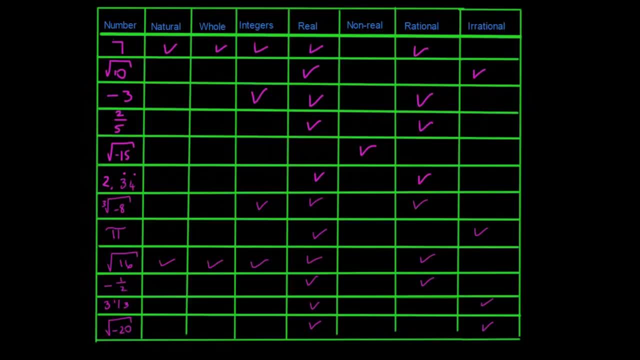 your own as well. Okay, so here we have a table. The table, if you look at our headings, it's our natural numbers, whole numbers, integers, real numbers, non-real numbers, rational numbers and irrational numbers. Those are our headings. And let's look at the first number. We've got number seven. So what? I? 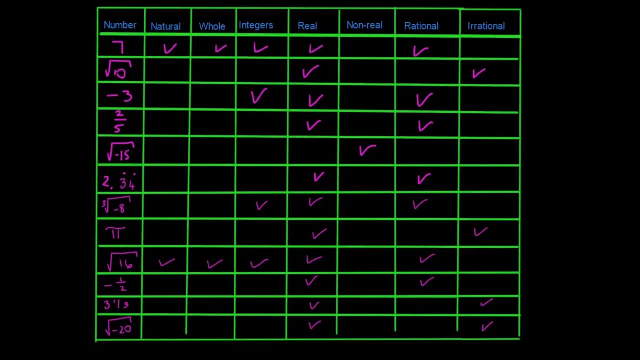 would like for you to be able to do. I'll do the first two with you. What you can do after that is: you can pause the video, Write down the numbers in the comment section below, And then you can click on the subscribe button, And then you can. 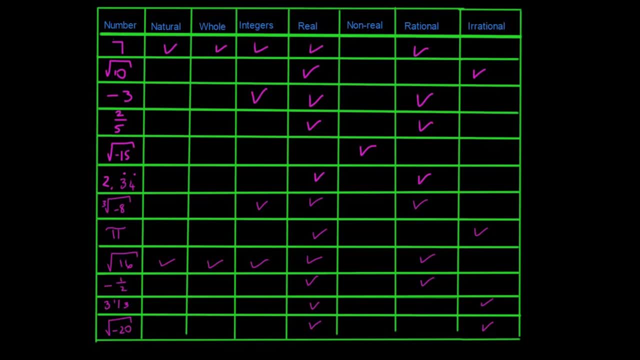 go to the column and then see if you can complete the table for yourself And then check it when you are done. Let's look at number seven. Number seven, it's a natural number, It's a whole number, It's an integer, It's a real number And it's a rational number. Remember we spoke about on the previous. 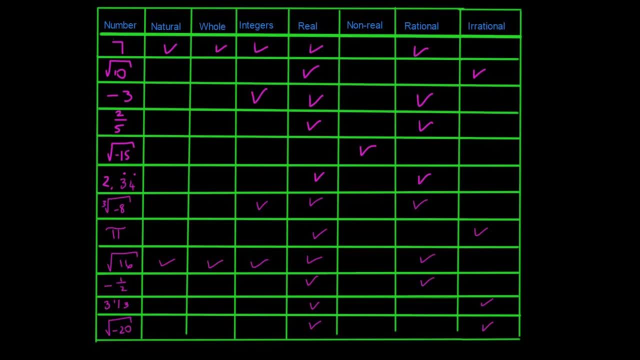 page we spoke about what those numbers are. Okay, if a number is real, it won't be non-real. Okay, they cannot be both. So numbers are either real or they're non-real. They're either rational or irrational. They won't be both, So they can be real and 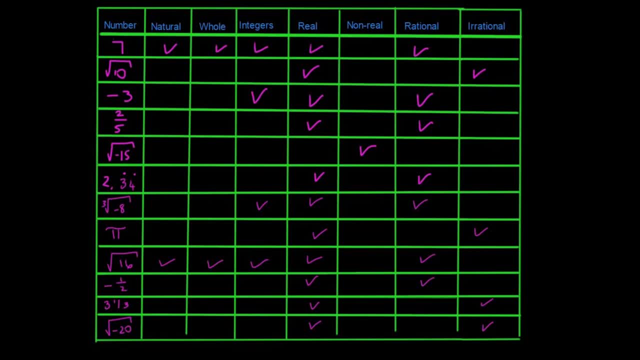 rational. They can be real and irrational, But they can't be real, rational and irrational. It must be real and rational or real and irrational. Okay, So let's have a look at the square root of 10.. The square root of 10, that is a real number. However, it's not a whole number. 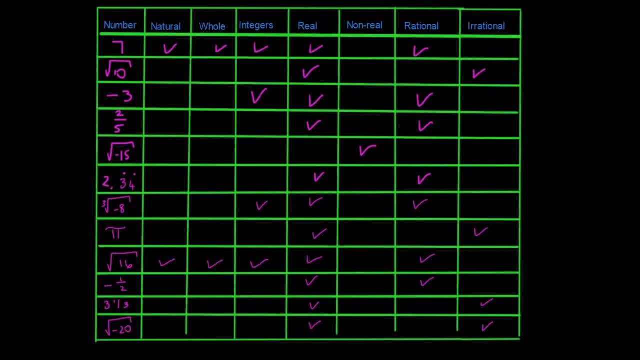 It's not a natural number, It's not an integer- Okay, Now it's a real number, but because it's the square root of a non-square number, it is irrational. Okay, so let's pause the video and take down the numbers that you see in front of you. 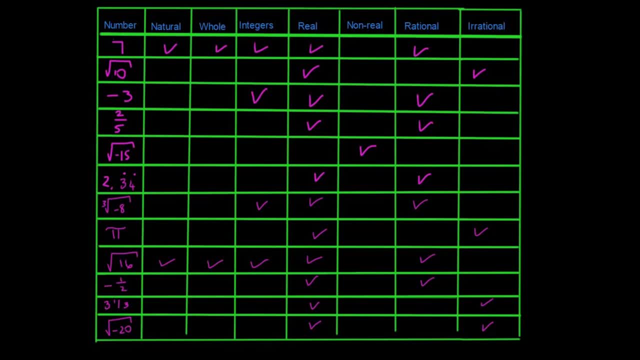 Take down the table and see if you can complete the rest by yourself, and we'll go over it and mark Okay. so we're back. Let's look at negative 3.. Negative 3 is an integer. Why is it not a natural number or a whole number? 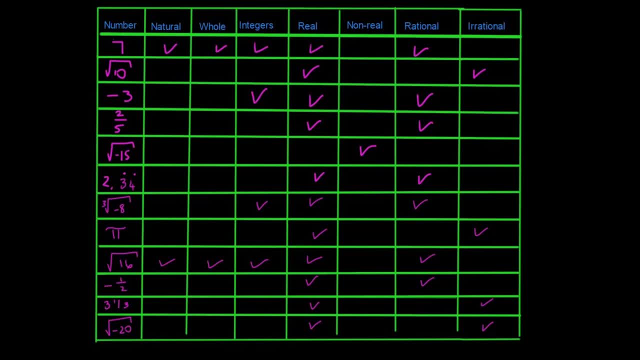 It's not a natural or a whole number, because these are only positive numbers. However, integers include negative numbers, So it's an integer, it's a real number and it's a rational number. Two-fifths: Remember we said that fractions, any number that is a fraction, is considered a rational number. 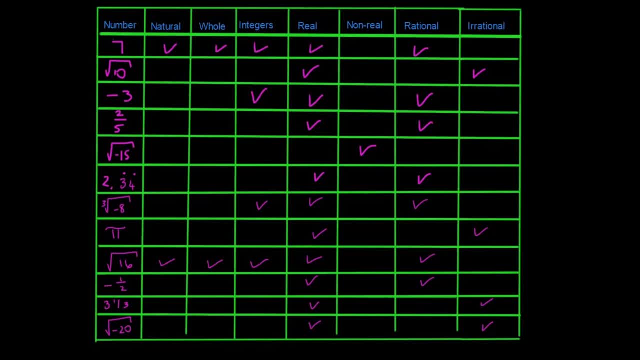 So it's a. It's a real number and it's a rational number. Let's look at the square root of negative 15.. What did we say about the square root of a negative number? We said that it is non-real. 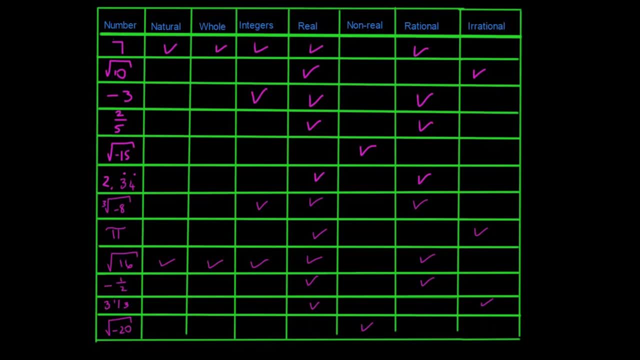 Now let's look at 2,34 recurring. There we have a recurring decimal. Recurring decimals are real and they are rational. Let's look at the next one, The cube root of negative 8.. Now, what's expected of you here? 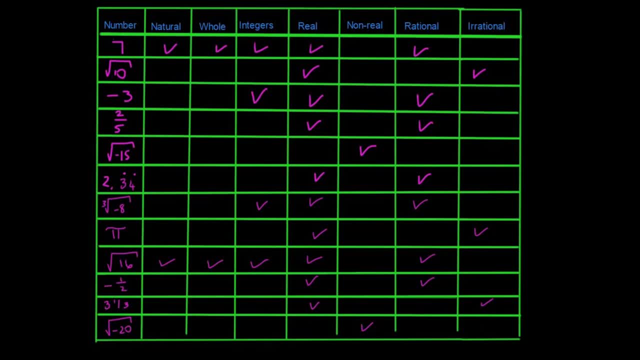 Here is for you to actually work out the answer. What is the cube root of negative 8?? It's negative 2.. And then we work with negative 2.. Negative 2 is an integer, it's a real number and it is a rational number. 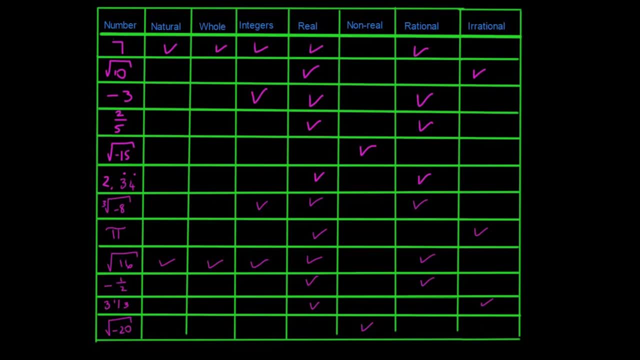 Let's look at pi, which we spoke about earlier. You've done it in error and perimeter. Pi is a real number, but it's also a non-terminating decimal, In other words, it doesn't end, And that makes it irrational. 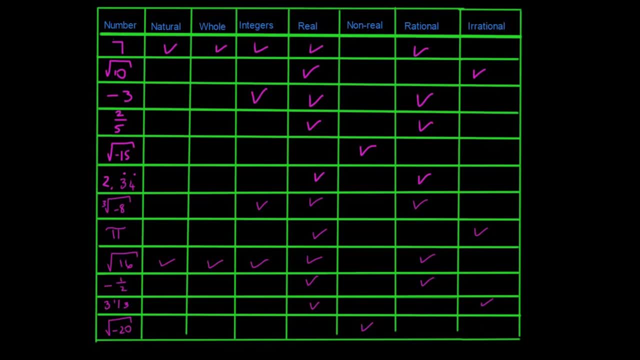 The next one, square root of 16.. Again, we need to work out the solution. Square root of 16 is 4, making it a natural number, a whole number, an integer, a real number as well as a rational number. 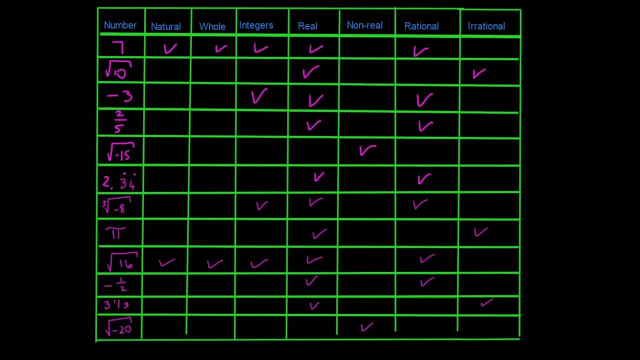 Negative: a half Written as a fraction. What do we know about fractions? They are real and they are rational. Let's look at three and a third. So you're going to say to me that three and a third is well, a third is a recurring decimal.